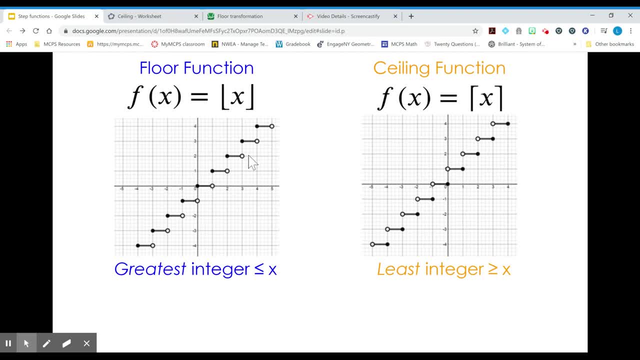 that are only integers For a floor function. the solid dot is on the left side and for any value, we are rounding down to the greatest integer less than or equal to that number. When x is 1.5,, our function equals 1.. When x is 2,, our function equals 2.. This is represented. 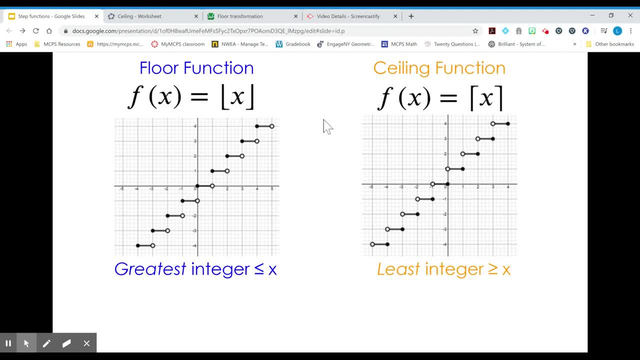 by a bracket that has a floor on it, which I like to think of as little feet For a ceiling function. our solid dot is on the right side and we are always rounding up to the least integer greater than or equal to that value. So now we have. 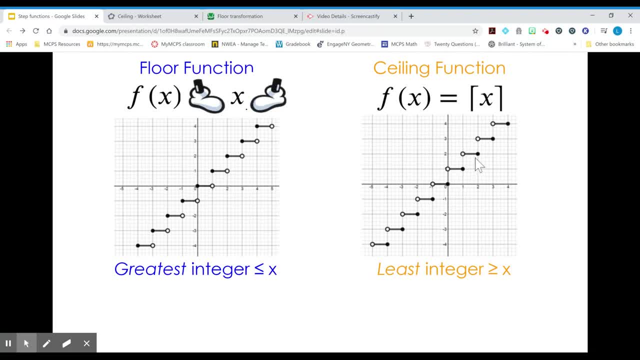 an x value of .5, and we are rounding up to 1.. This is represented in our notation by a bracket with a ceiling on it. We can use our graph to evaluate our function for any particular value For a floor function. we are always rounding down. 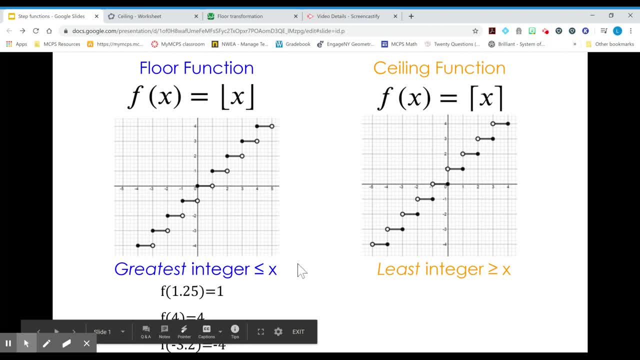 to the least integer greater than or equal to that value. Our function for a particular integer equals that integer. And note: for a negative number, negative 3.2 is rounded down to the greatest integer less than that. so it is rounded down to negative 4.. For our 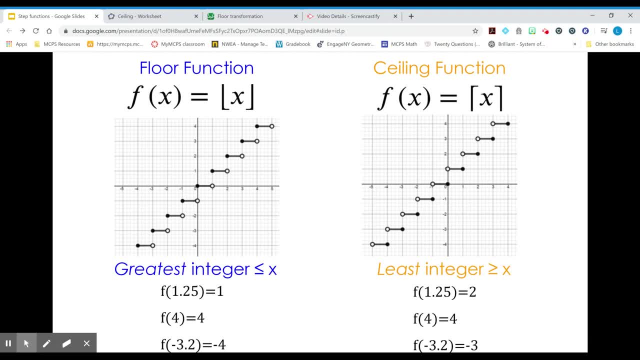 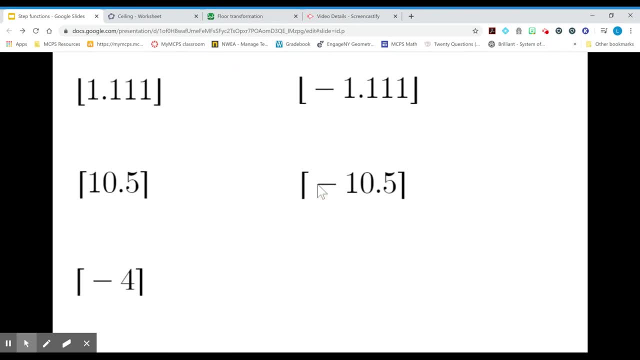 ceiling function. you can see that we are rounding up and negative 3.2 rounds up to negative 3.. Pause this video and evaluate these expressions. Notice whether you are evaluating a floor function or a ceiling function. The first two are floor functions, so we are rounding down to the greatest, integer less. 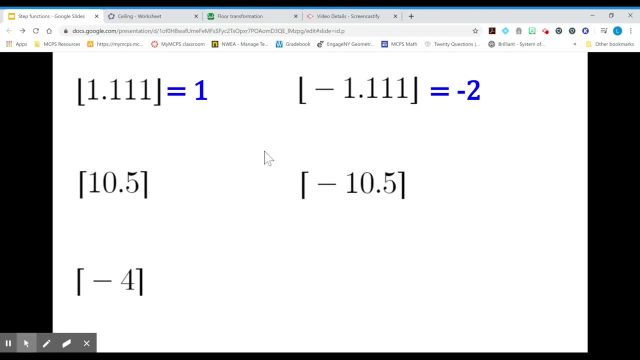 than or equal to that number. The next two are ceiling functions. so we are rounding up to the least integer greater than those numbers. Lastly, the ceiling function of negative 4 equals negative 4.. I want to take a moment and explore the transformations of step functions. Notice that the transformations 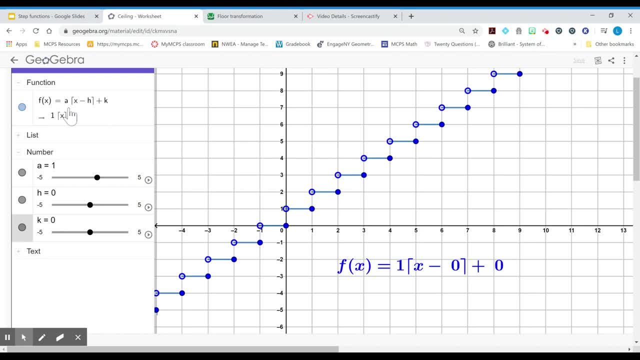 are represented in the same way you learned about the transformations for quadratic functions. A is our vertical dilation. A increases the distance between our steps. When A is between 1 and negative- 1,- our steps get closer together, And when A is negative, we have: 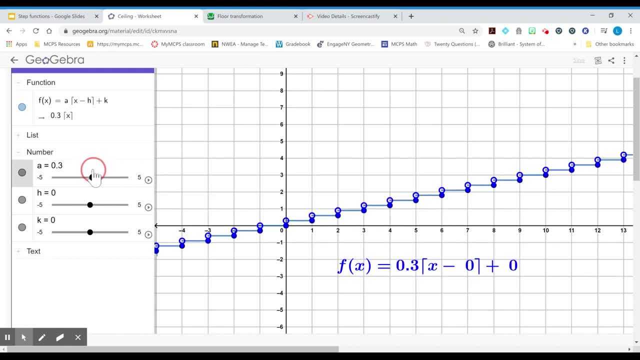 a reflection across the x-axis. H shifts our function right or left. It is our horizontal translation. So when x is positive, we have a translation to the right and you can see that represented in our equation. K shifts our function up or down. It is our vertical translation And again you can see. 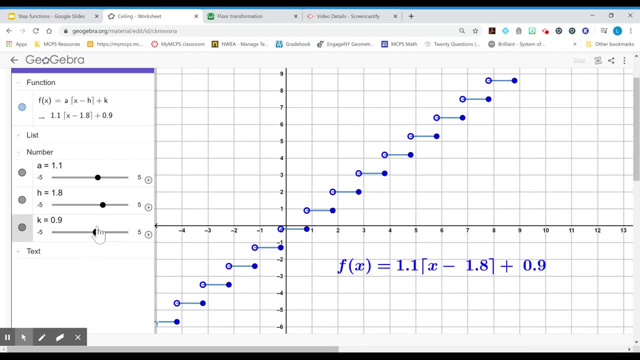 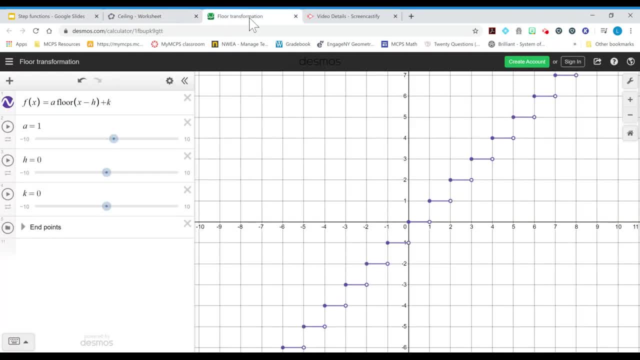 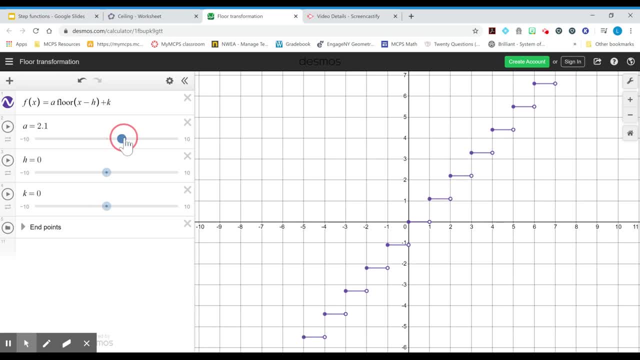 dot is on the left side. when we are rounding down, You can see that A has the same impact. Even if A is negative, the solid dot is still on the left side And H shifts our equation left or right And K shifts our function up or down. 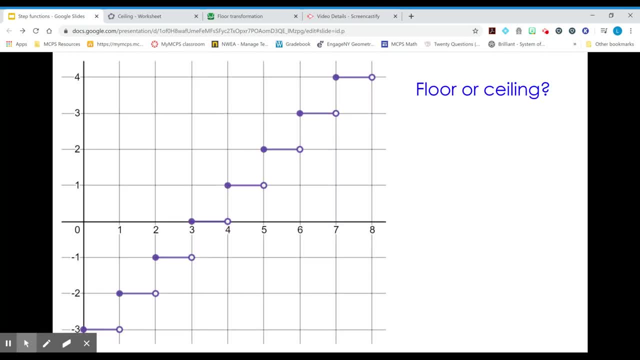 Pause the video again and evaluate whether this is a floor function or a ceiling function and what transformations have occurred. Pause the video again and evaluate whether this is a floor function or a ceiling function and what transformations have occurred. This is a floor function because our solid dot is on the left side, meaning we are rounding. 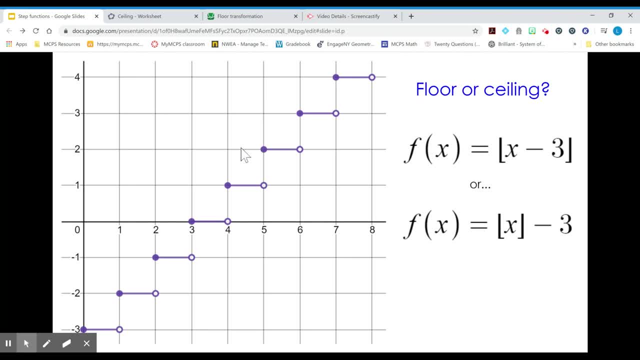 down. Our A value is 1, because our steps are one unit apart. We can write this either as a horizontal translation, three units to the right, by subtracting an H value of 3.. Or Or we can write it as a vertical translation, three units down, by adding a k value of negative three. I hope you have enjoyed this video.